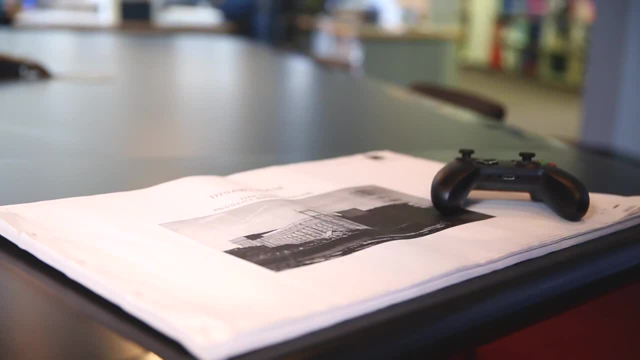 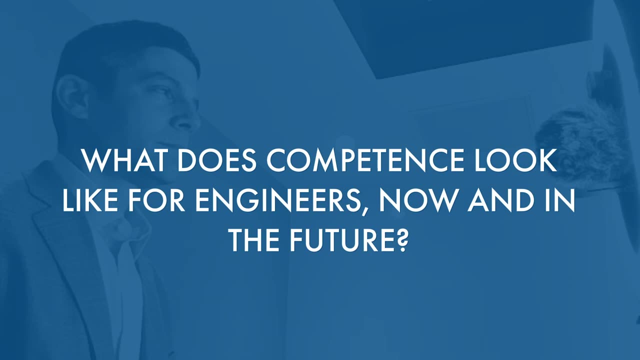 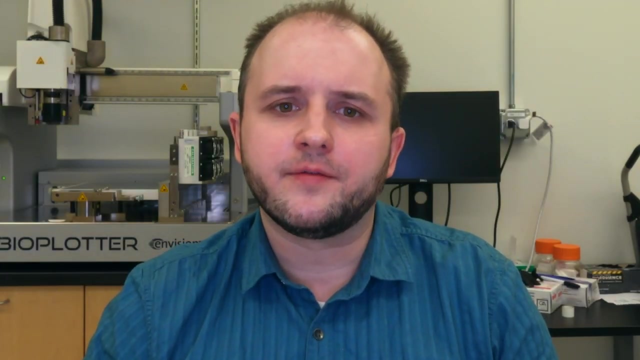 i'm not really sure, but i think this is okay. that's really never okay. the idea of confidence is going to change quite a bit in terms of it's going to become more specialized. so what i think is going to happen is they're going to be more certification programs for 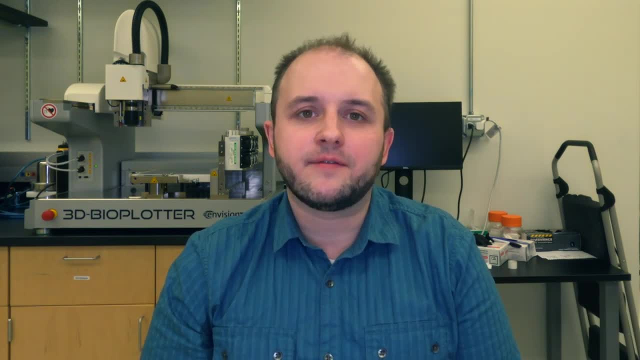 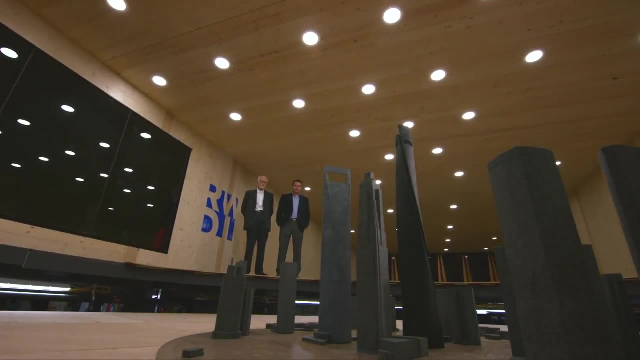 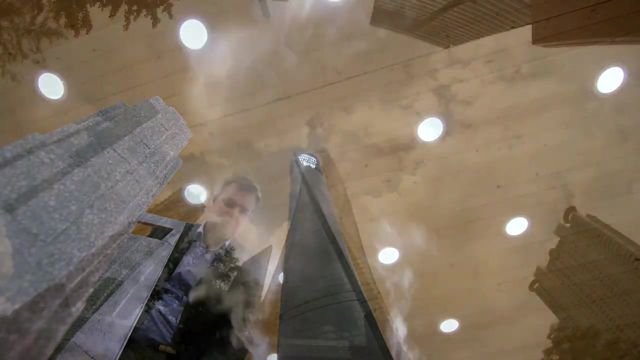 really specific applications of engineering. that helps kind of establish competency. i think we have to kind of take our careers on a parallel path. on the one hand we have to take a very high level in general view of engineering science, but at the same time, on a parallel path, we need to be able: 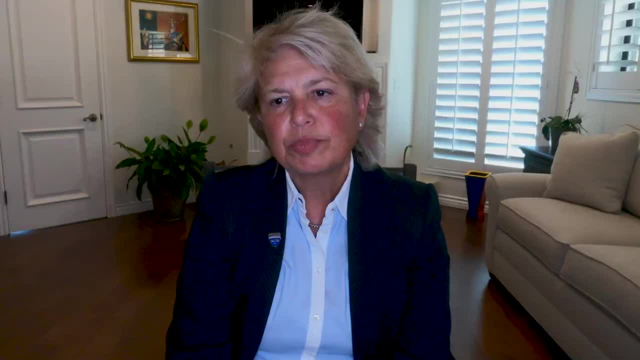 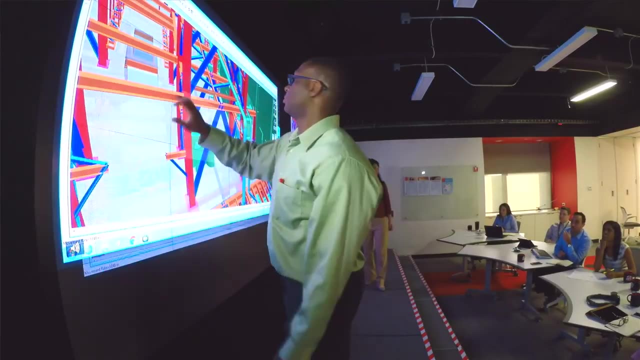 to take deep dives into our areas of expertise. problems need to be solved in a team model, where you bring in different experts from different fields that all come together towards an integrated project. the pieces of the charm of engineering that we have to take a deep dive into, such as the 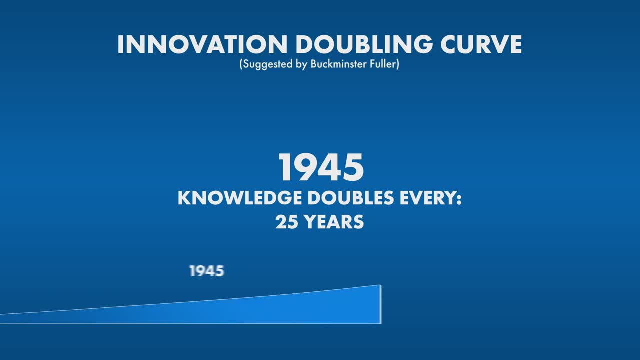 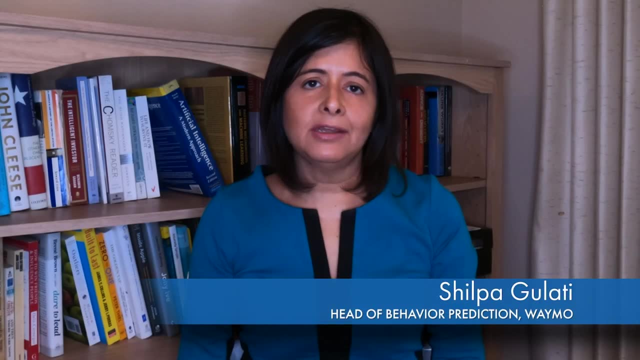 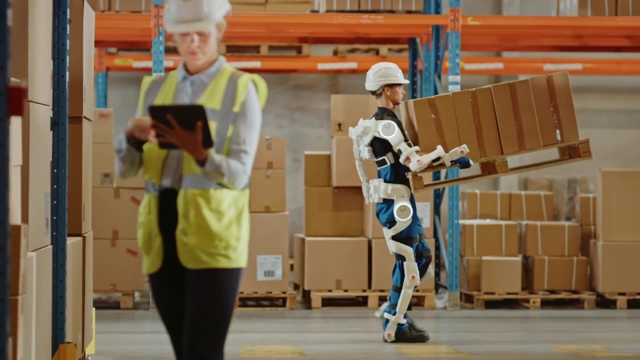 The pace of innovation is accelerating and new knowledge is being constantly created. Therefore, we cannot stand on the knowledge that we learned in the past. We have to be on our feet and continuously learn. Engineers push innovation forward because we think differently. We try to push the limit of what the human body, what the next machine can do. 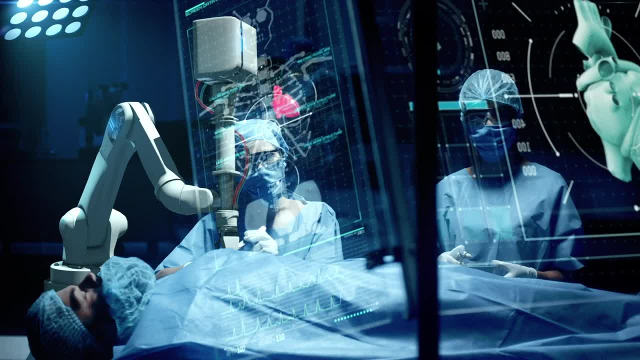 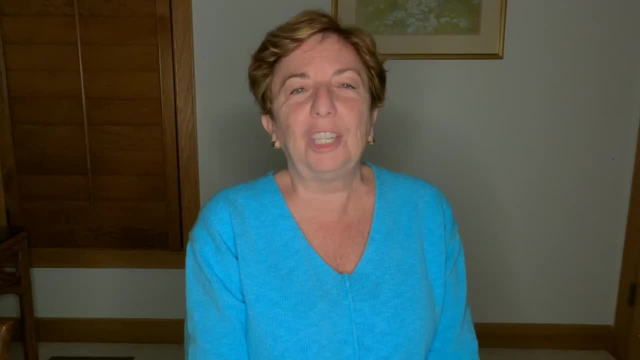 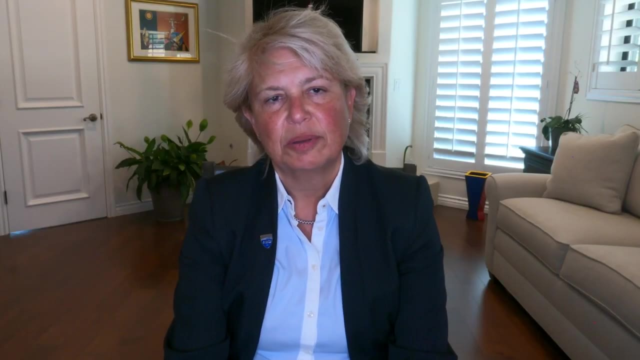 So the pace of innovation is expanding really rapidly, exponentially even. And I say this because, you know, 10 years ago the field I'm in now didn't exist. Engineering knowledge is supposed to be doubling every 13 months. Well, the pace of innovation is mind-boggling. 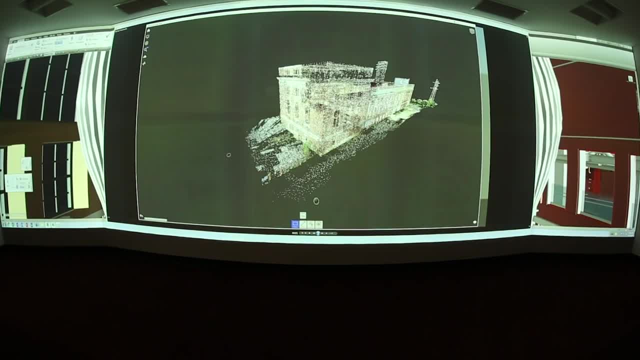 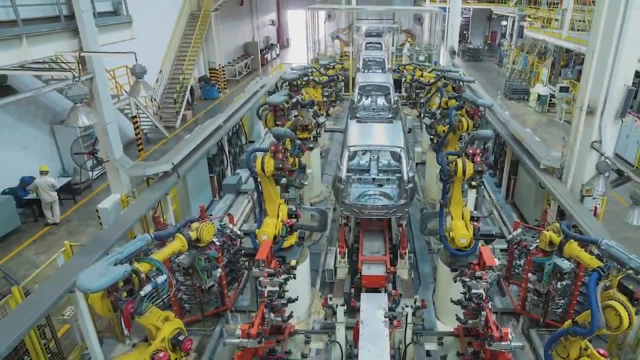 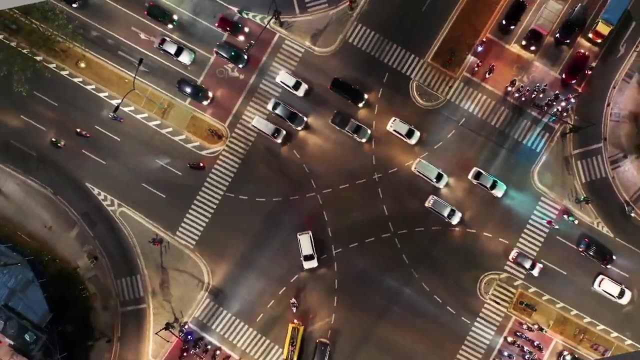 Our government agency is trying to keep up with the many developments that are currently out in the market: Robotics and construction, robotics and manufacturing artificial intelligence, autonomous vehicles, which will change the way we design our transportation Infrastructure, the need for a broad-based telecommunications infrastructure and everything. 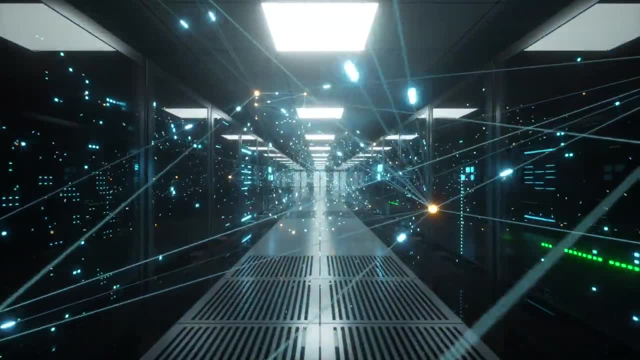 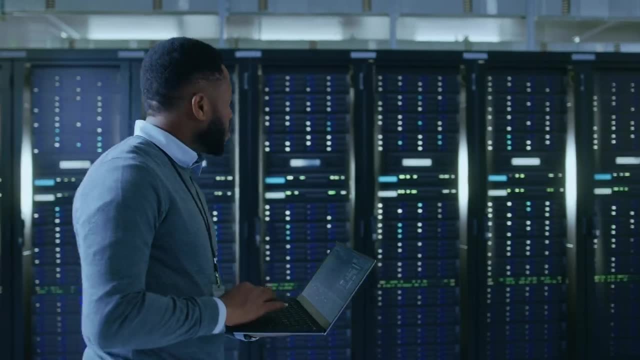 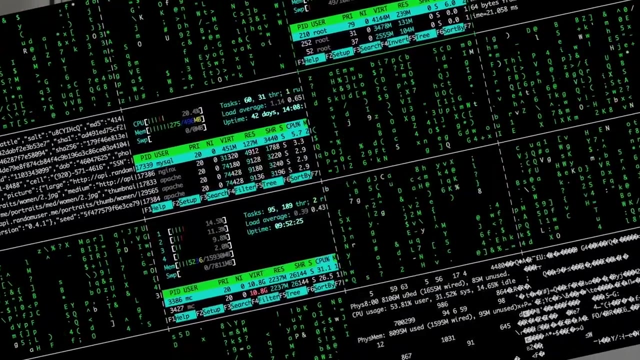 that comes with the integration of all these systems. that's what's so exciting and challenging at the same time. It is the engineer's ethical duty to understand the algorithms that we develop, the data that's being put into those algorithms and the outputs of those algorithms, because it can be a disastrous.